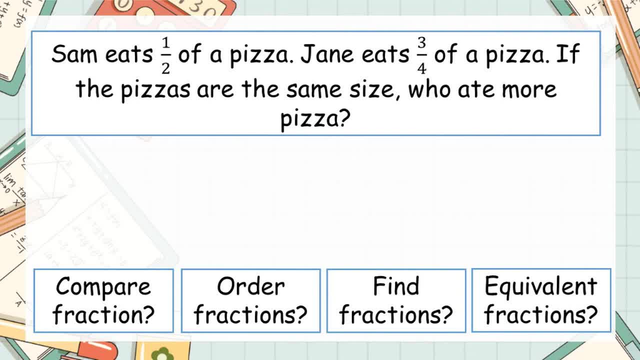 We know how to compare fractions, how to order fractions, how to find fractions of sets and how to find equivalent fractions. We did all them during the week. We just need to figure out which type of question this one is. So let's have a look at it again. Sam eats one half of a pizza. Jane eats three quarters of pizza. Who ate more? 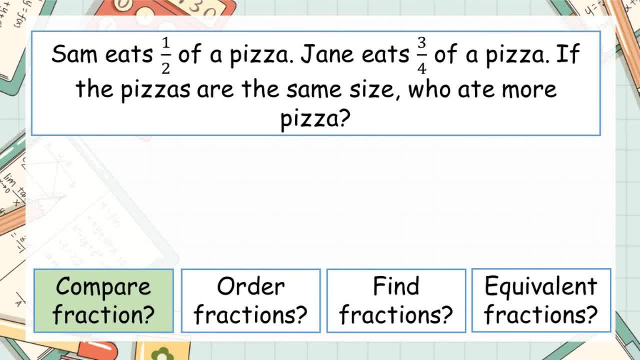 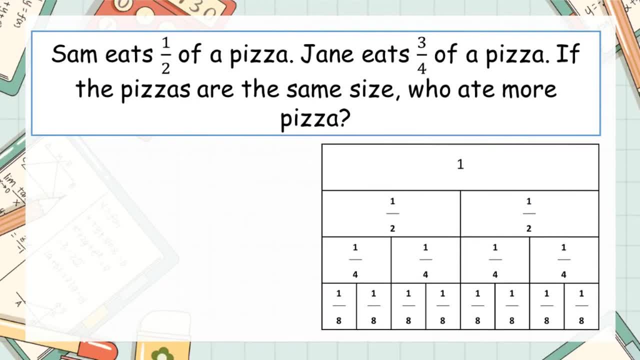 Ah, so they're asking us to compare two fractions to see which one is larger: One, half or three quarters. Can you use the fraction wall here to help you find the answer to this word problem? Remember, we're trying to find which one of these two fractions is bigger. 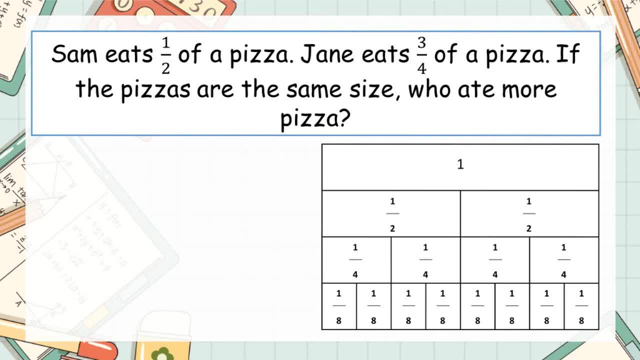 That will tell us who ate more pizza. Pause the video and give it a try. Well, if we take a look at those two fractions on the fraction wall- one half and three quarters- we can see that three quarters is bigger. So, Jane, ate more pizza? That's our answer, Jane. Let's try another one with a different type of problem. 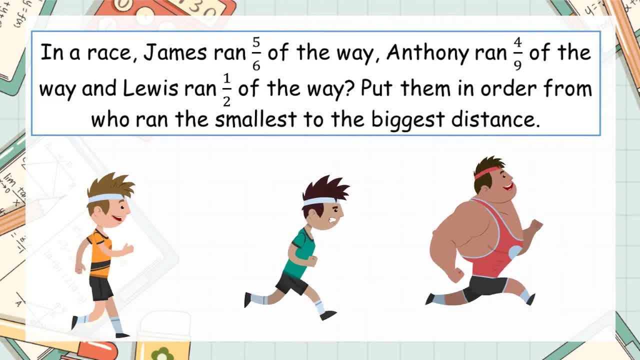 we have some people running in a race. So in a race, James ran five-sixths of the way, Anthony ran four-ninths of the way and Lewis ran half of the way. Put these in order from who ran the smallest to the biggest distance. So again we need to try figure out what kind of question is. 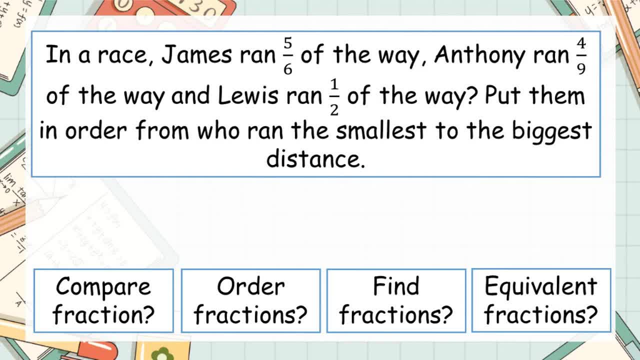 this: Is it a comparing, an ordering, a finding, or is it an equivalent fraction question? Pause the video and see if you can figure out which one of these four types of question it is. Well, did you get it correct? This is, of course, an ordering fractions question. The clue is in: 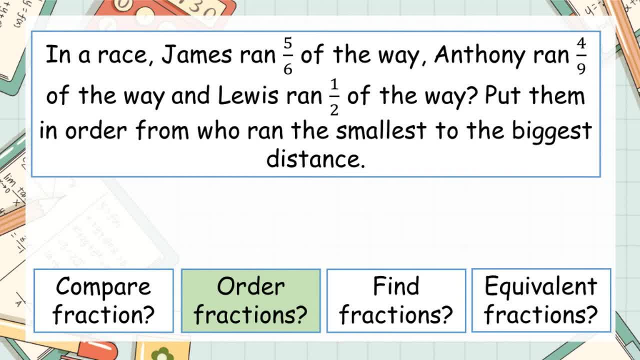 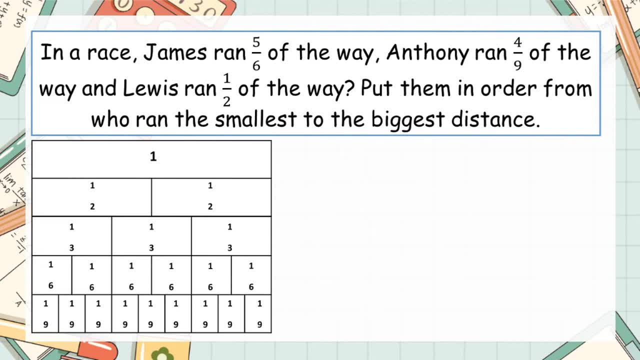 the question. It says: put them in order. Here's a fraction wall that will help you solve this question. Use the fraction wall To help you find the answer to the problem above. Pause the video and write down your answer. Well, how did you get on When we color in those fractions and take a look at them? on the fraction. 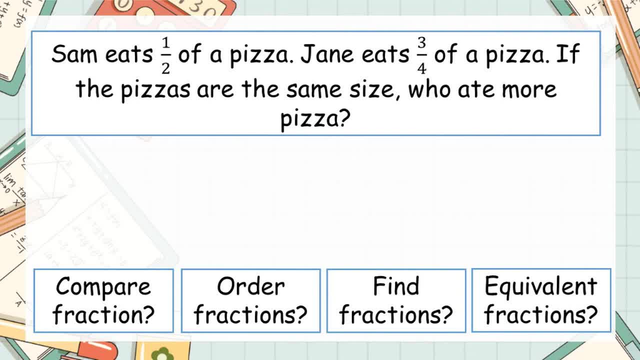 We know how to compare fractions, how to order fractions, how to find fractions of sets and how to find equivalent fractions. We did all them during the week. We just need to figure out which type of question this one is. So let's have a look at it again. Sam eats one half of a pizza. Jane eats three quarters of pizza. Who ate more? 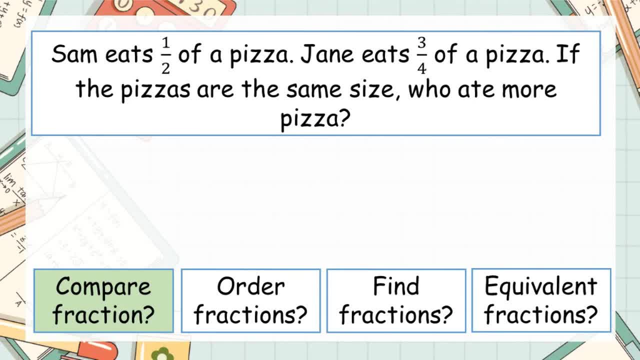 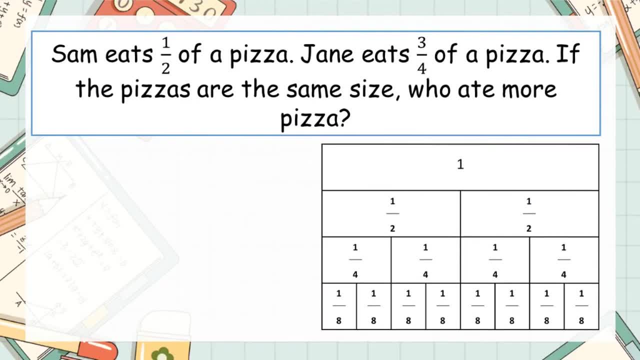 Ah, so they're asking us to compare two fractions to see which one is larger: One, half or three quarters. Can you use the fraction wall here to help you find the answer to this word problem? Remember, we're trying to find which one of these two fractions is bigger. 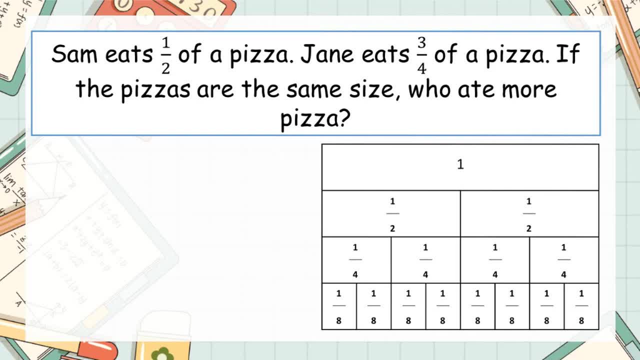 That will tell us who ate more pizza. Pause the video and give it a try. Well, if we take a look at those two fractions on the fraction wall- one half and three quarters- We can see that three quarters is bigger. So, Jane, ate more pizza? That's our answer, Jane. Let's try another one with a different type of problem. 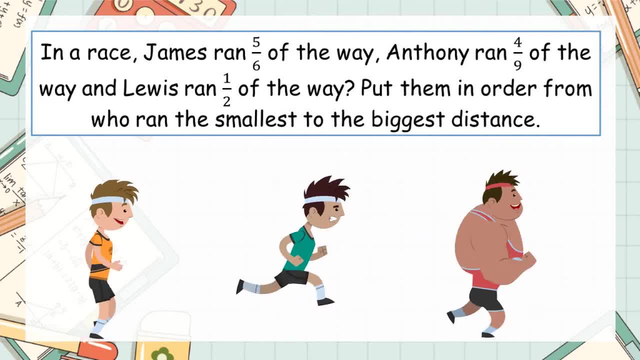 problem Here. we have some people running in a race. So in a race James ran five sixths of the way, Anthony ran four ninths of the way and Lewis ran half of the way. Put these in order from who ran the smallest to the biggest distance. So again we need to try figure out what kind of question. 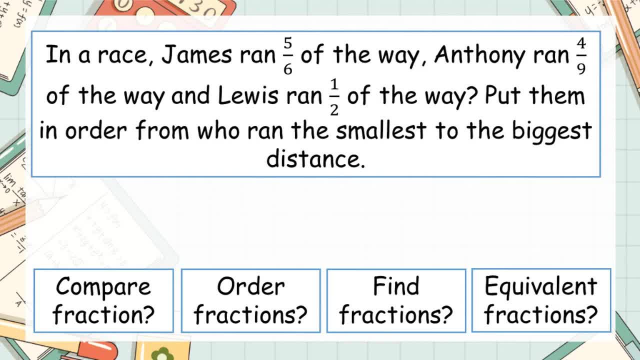 is this? Is it a comparing, an ordering, a finding, or is it an equivalent fraction question? Pause the video and see if you can figure out which one of these four types of question it is. Well, did you get it correct? This is, of course, an ordering fractions question. The clue is in the 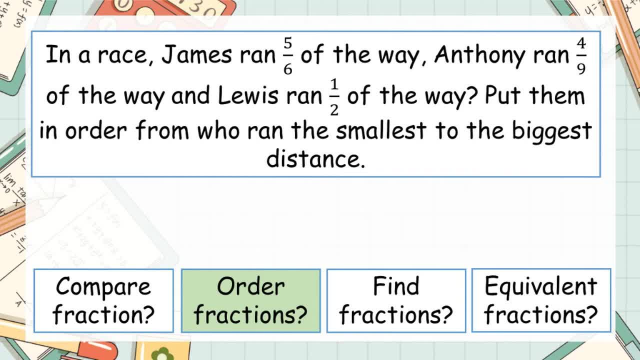 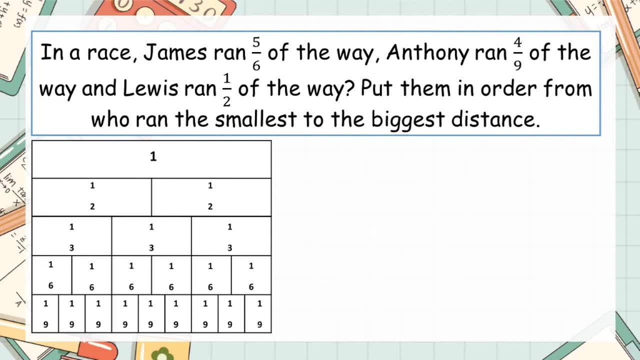 question. It says: put them in order. Here's a fraction wall that will help you solve this question. Use the fraction wall to help you find the answer to the problem above. Pause the video and write down your answer. Well, how did you get on When we color in those fractions and take a look at them? 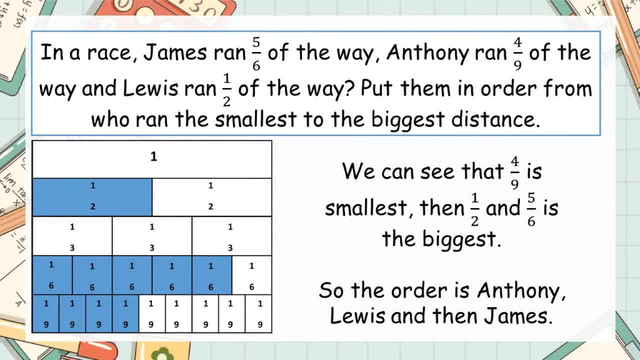 on the fraction wall we can see that four ninths is the smallest value, then one half and finally five sixths is the biggest. So the order is Anthony, Lewis and then James. Did you get that one correct? Here comes the next question At lunchtime. 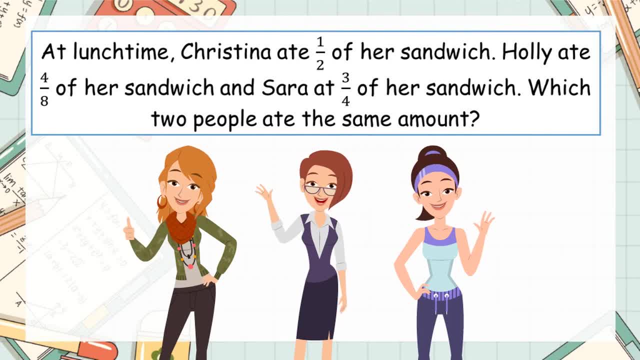 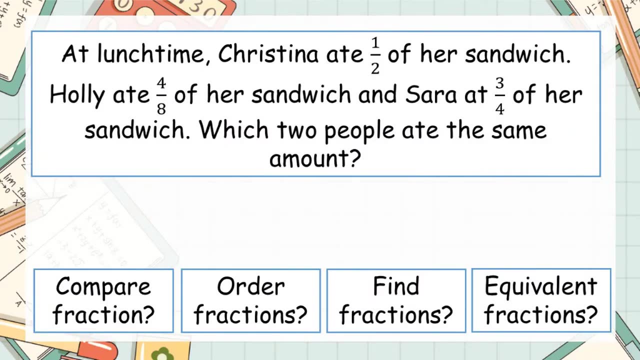 Christina ate half of her sandwich, Holly ate four eighths of her sandwich and Sarah ate three quarters of her sandwich, Which two people ate the same amount. Okay, so again, what kind of question is this? Is it a comparing, an ordering? 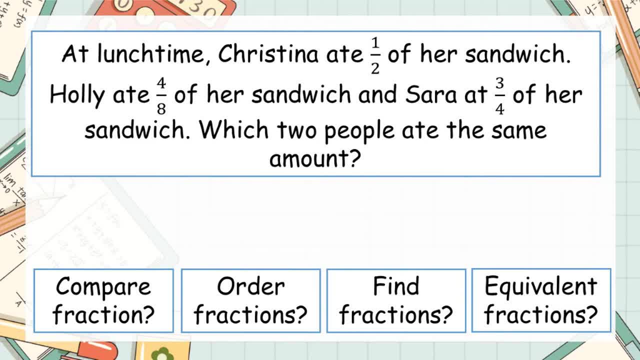 finding fractions or is it an equivalent? Pause the video and see if you can figure out which type of question it is. Well, this is an equivalent fraction question. Remember those ones where we see which fractions are equal to each other. Use the fraction wall down below to help you solve the word. 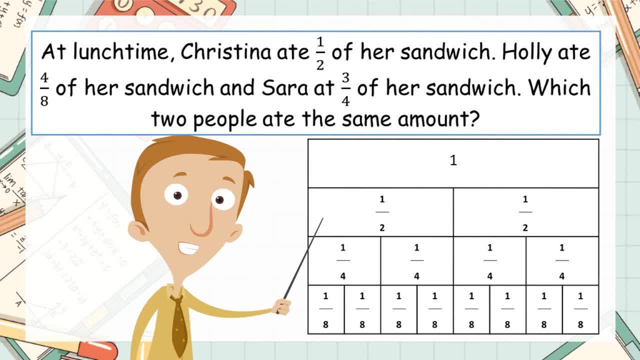 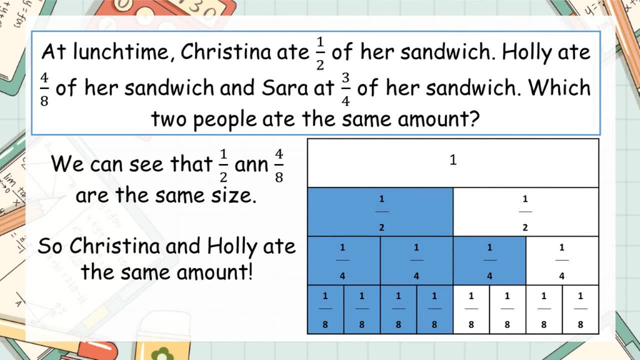 problem. Remember, you're looking for the two people who ate the same amount, So you're looking for which two fractions are equivalent. Pause the video and give it a try. Well, when we put these all onto the fraction wall, we can see that one half and four eighths are the same size. 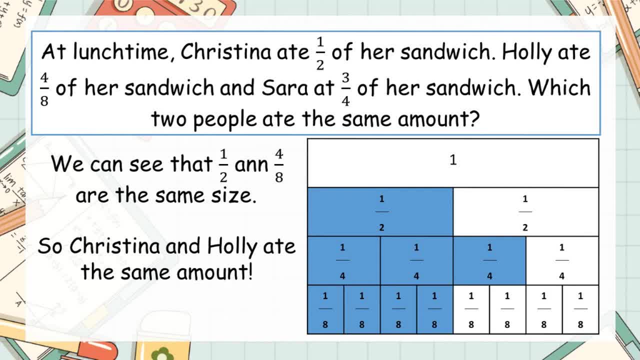 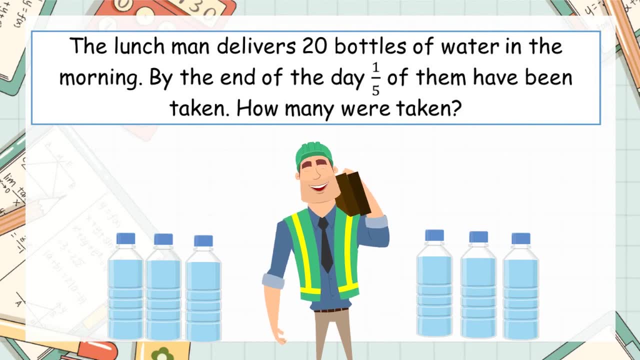 So Christina and Holly ate the same amount. Okay, now let's go on to the next question type. In my opinion, this is the hardest of all fraction questions that you'll come across in fourth class, But I'll leave it up to you to decide. So our question is: the lunch man delivers 20 bottles of water in the morning. By the end of the day, one fifth of them have been taken. How many were taken? 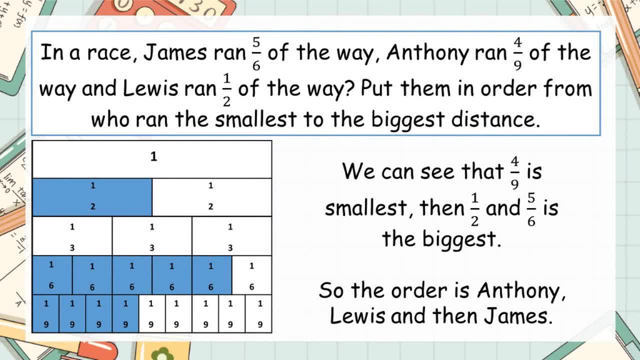 wall we can see that four-ninths is the smallest value, then one-half and finally five-sixths is the biggest. So the order is Anthony, Lewis and then James. Did you get that one correct? Here comes the next question. 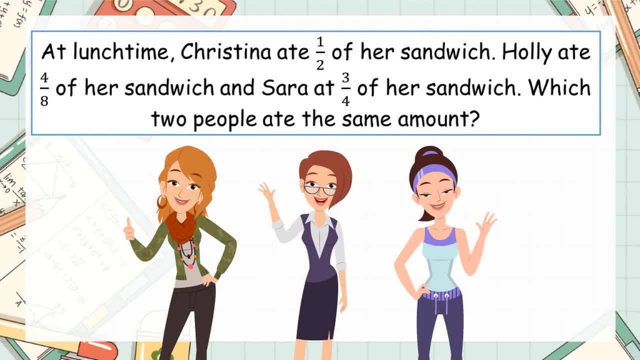 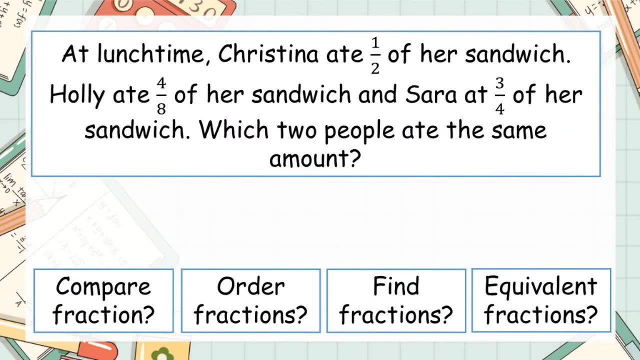 At lunchtime. Christina ate half of her sandwich, Holly ate four-eighths of her sandwich and Sarah ate three-quarters of her sandwich, Which two people ate the same amount, Hmm, okay. so again, what kind of question is this? Is it a comparing, an ordering? 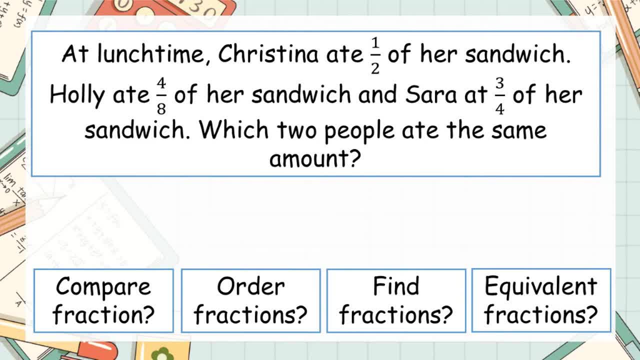 a finding fractions or is it an equivalent? Pause the video and see if you can figure it out. it an equivalent? hmm, pause the video and see if you can figure out which type of question it is. well, this is an equivalent fraction question. remember those ones where we see which fractions are equal to each other. use the fraction. 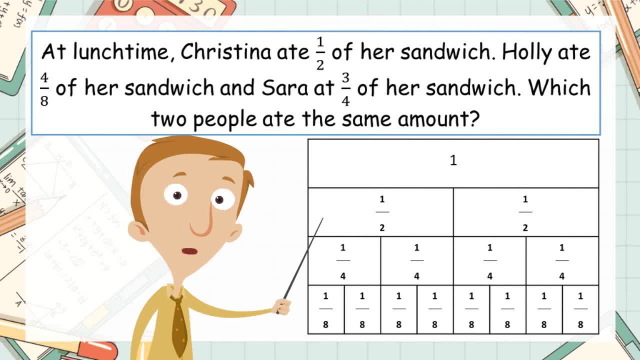 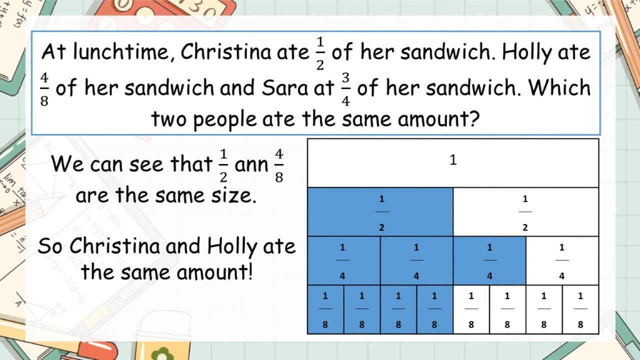 wall down below to help you solve the word problem. remember, you're looking for the two people who ate the same amount, so you're looking for which two fractions are equivalent. pause the video and give it a try. well, when we put these all onto the fraction wall, we can see that one half and four eighths are. 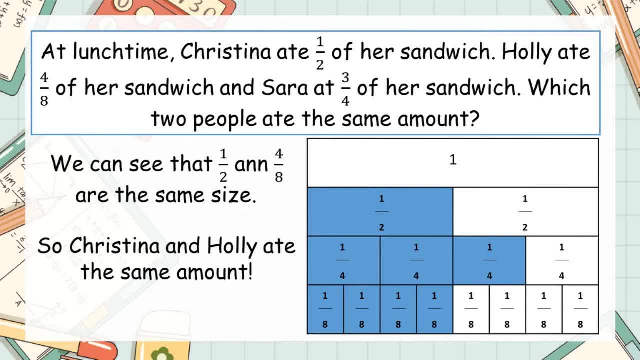 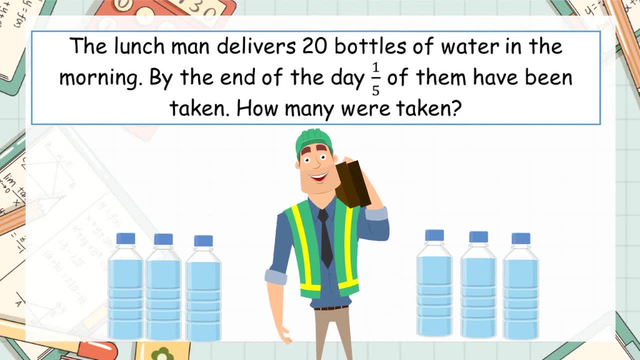 the same size, so Christina and Holly ate the same amount. okay, now let's go on to the next question type. in my opinion, this is the hardest of all fraction questions that you'll come across in fourth class. boss, I'll leave it up to you to decide. 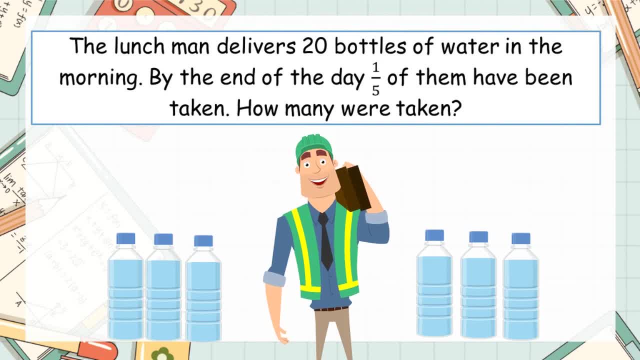 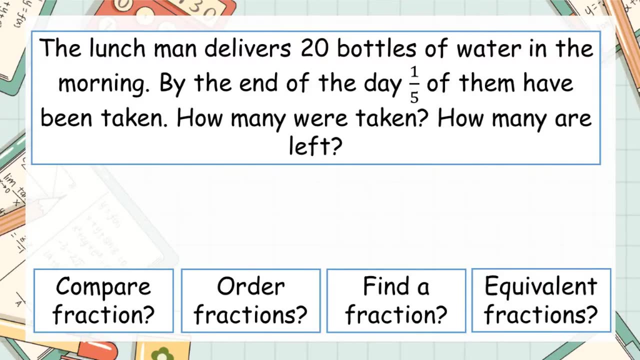 so our question is: the lunch man delivers 20 bottles of water in the morning. by the end of the day, one-fifth of them have been taken. how many were taken? hmm, so is this a comparing question, an ordering question, a find, a fraction of a set question, or? 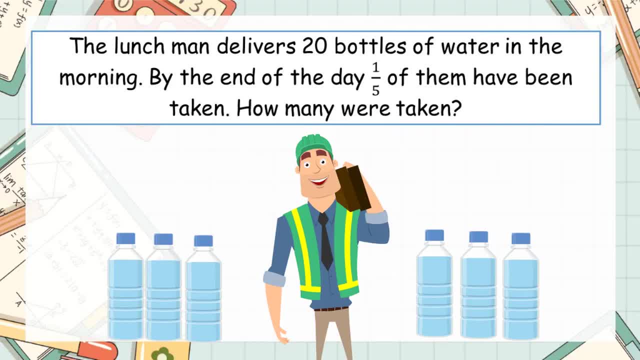 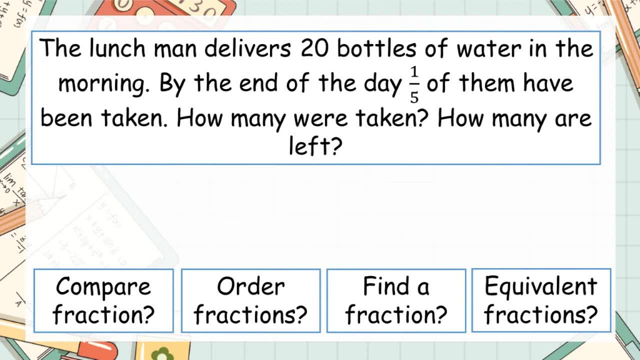 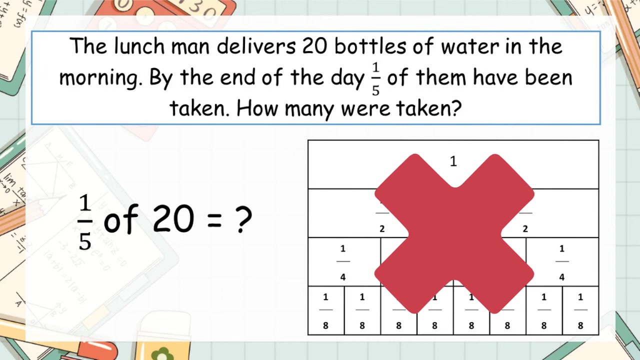 Hmm, So is this a comparing question, an ordering question, a find, a fraction of a set question or an equivalent fraction question? Pause the video and see which one it might be. Well, this is a find, a fraction of a set question. We did these last week, you might remember, So our fraction wall is not going to help us with this one. Unfortunately, there's no way we can use it to figure out what the answer is. Instead, we have to try and do a sum. 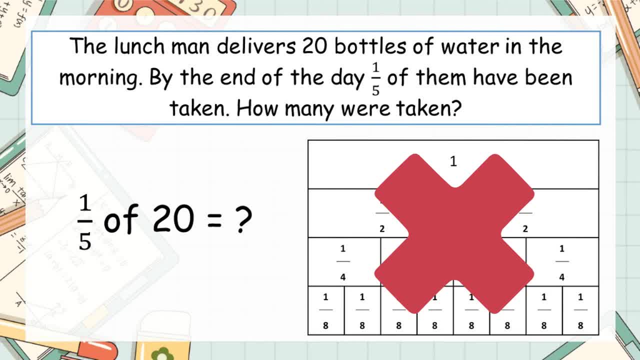 So remember these questions. Okay, one fifth of 20 is equal to something, So your answer should be: one fifth of 20 equals something. Can you remember how we solved that type of fraction problem? So your answer should be: one fifth of 20 equals something. 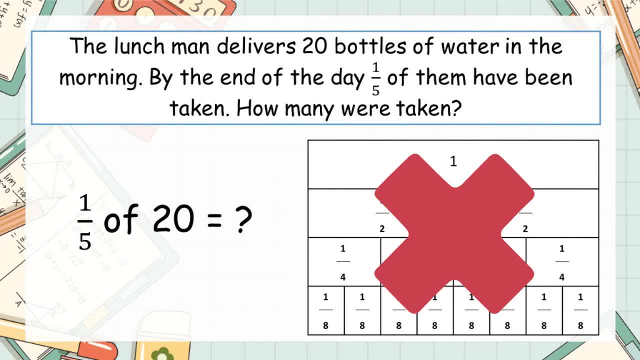 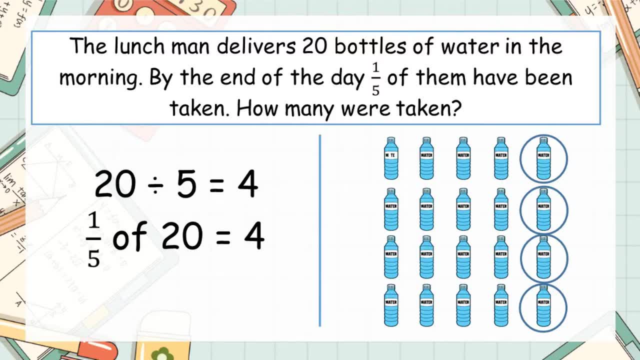 Pause the video and see if you can figure out what the answer is. Can you remember how we solved that type of fraction problem? Well, did you remember how we solved those? Remember there's two different ways we could have done it. I mean difficult. 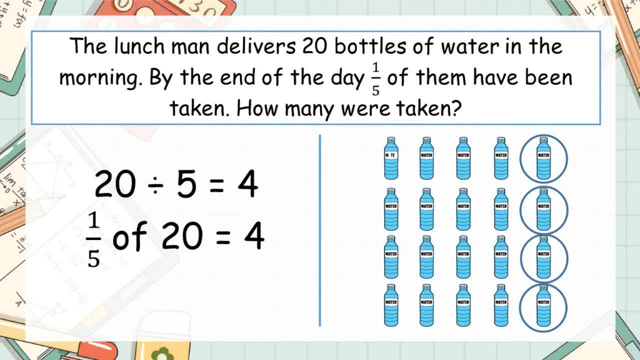 The first way involves division. We divide by the bottom number, We divide by the bottom number, We divide by the bottom number, denominator of the fraction. So 20 divided by 5 is equal to 4.. So one-fifth of 20 is equal to 4.. 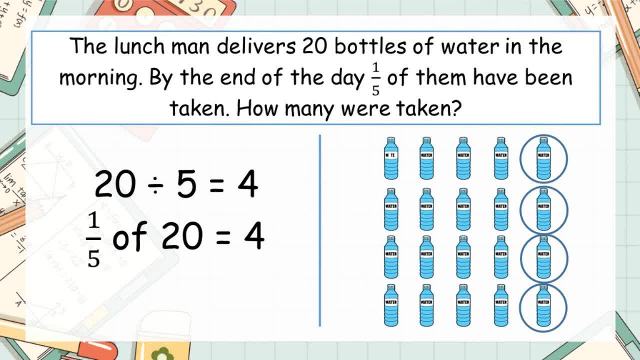 The other way we could have done it is by drawing a picture. If we drew out the 20 water bottles and we know that every 1 in 5 bottles have been taken, we count up 1,, 2,, 3,, 4, 5 and cross out. 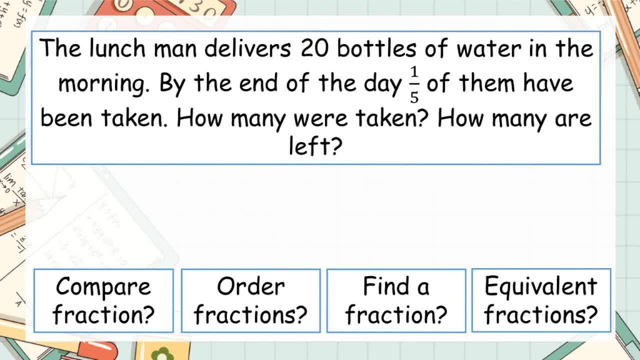 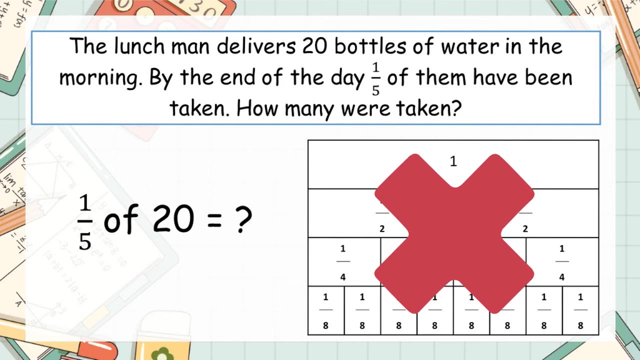 a equivalent fraction question. pause the video and see which one it might be. well, this is a find, a fraction of a set question. we did these last week, you might remember, so our fraction wall is not going to help us with this one, unfortunately. there's no way we can use it to figure out what the answer is. 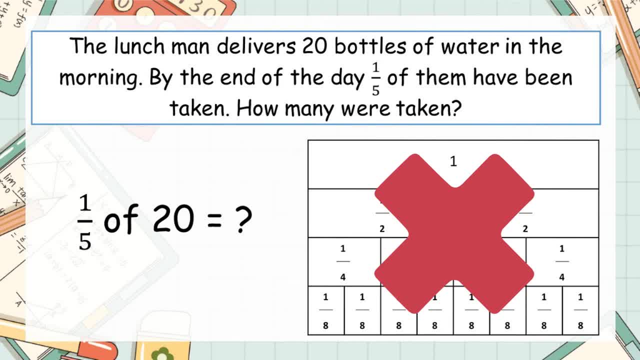 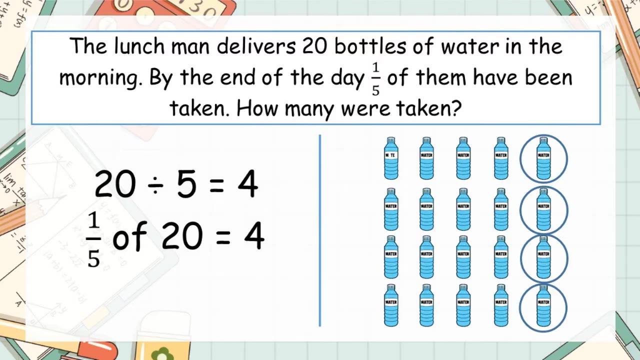 instead we have to try and do a sum. so remember these questions. one-fifth of 20 is equal to something. can you remember how we solve that type of fraction problem? pause the video and see if you can figure out what the answer is. well, did you remember how we solve those? remember there's two different ways. we 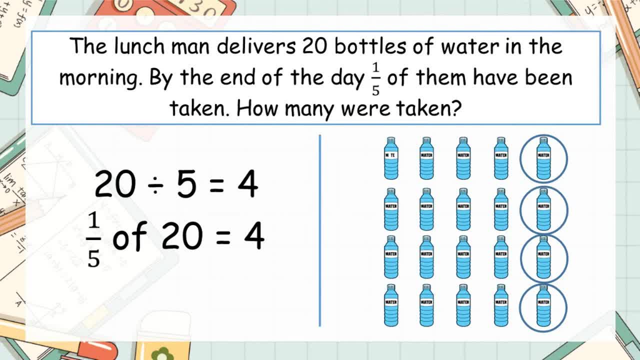 could have done it. the first way involves division. we divide and divide by the bottom number, the denominator of the fraction. so 20 divided by 5 is equal to 4. so one-fifth of 20 is equal to 4. the other way we could have done it is by: 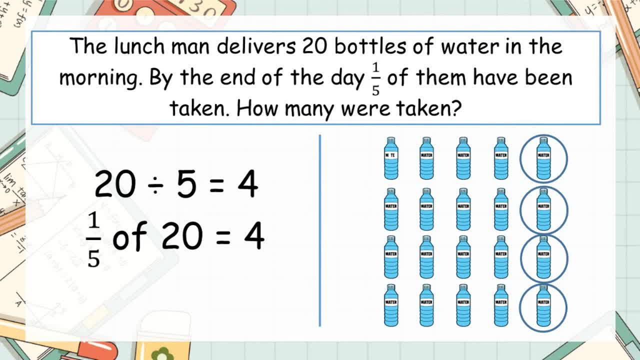 drawing a picture. if we drew out the 20 water bottles and we know that every one in five bottles have been taken, we count up 1, 2, 3, 4, 5 and cross out one of them. we We keep doing that until there's no water bottles left. 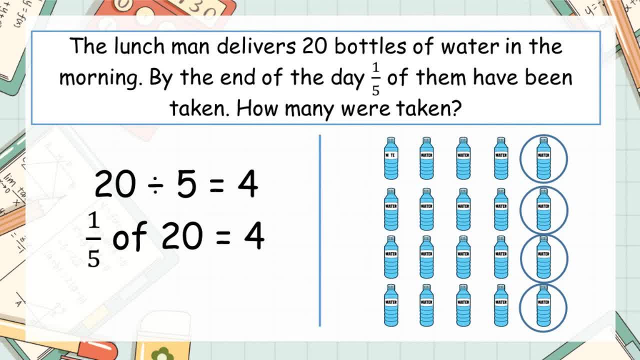 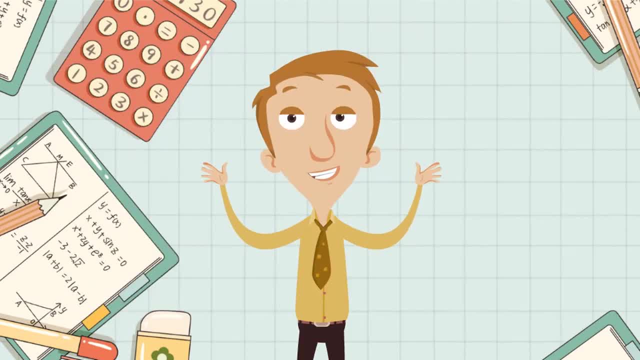 one of them. We keep doing that until there's no water bottles left And we would have got the same answer: 4 water bottles have been taken. Got all those correct. You are an absolute superstar at fraction word problems, because they were tricky. It's always hardest to try and figure. 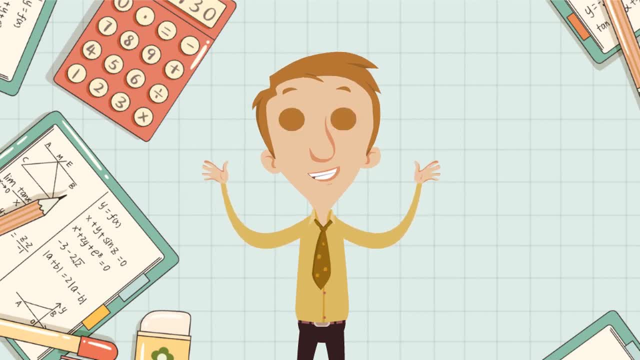 out what they want you to do in the word problem. For the last question type, this is the hardest type that you're going to see. These are actually questions, Kind of more 5th class maths, So give them a try and see if you can figure them out. 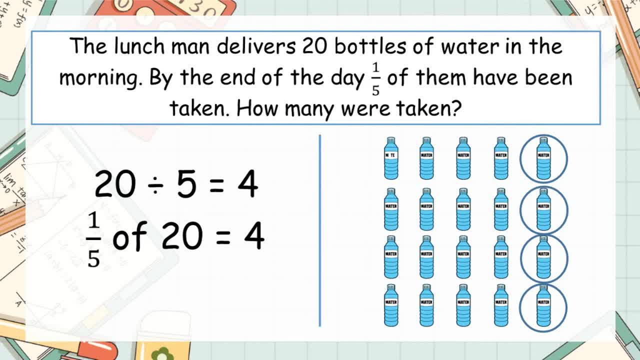 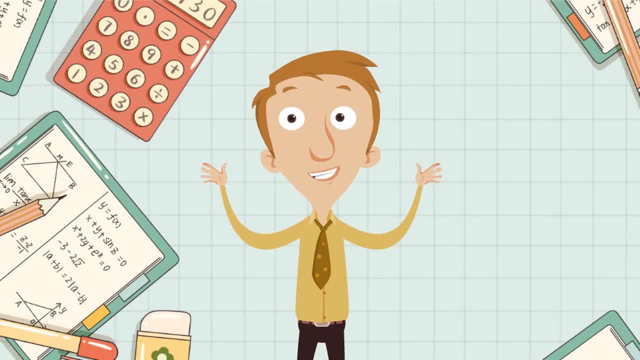 And we would have got the same answer. Four water bottles have been taken. Got all those correct. You are an absolute superstar at fraction word problems, because they were tricky. It's always hardest to try and figure out what they want you to do in the word problem. 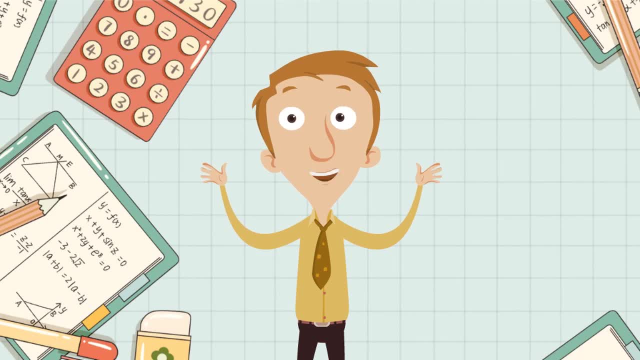 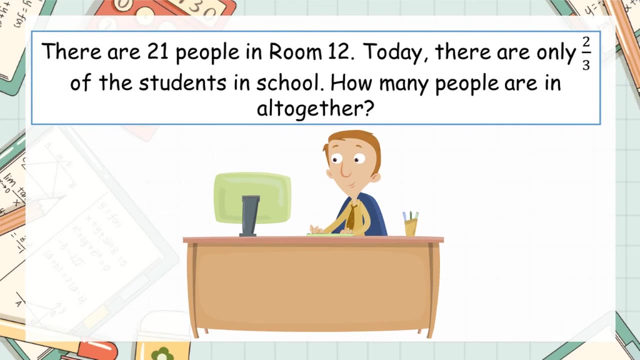 For the last question type. this is the hardest type that you're going to see. These are actually kind of more fifth class maths, So give them a try and see if you can figure them out. There are 21 people in room 12.. 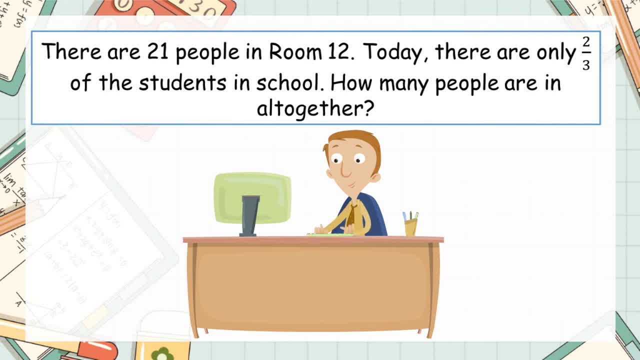 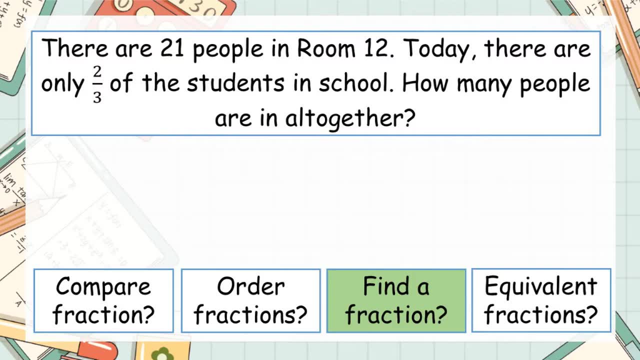 Today, there are only two thirds of the students in school. How many people are in altogether? Now, this is a finding, a fraction of a set question, Just like the last one we did, But there's one extra Step we have to do. 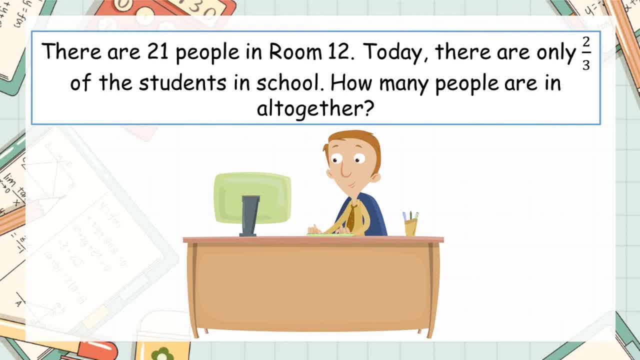 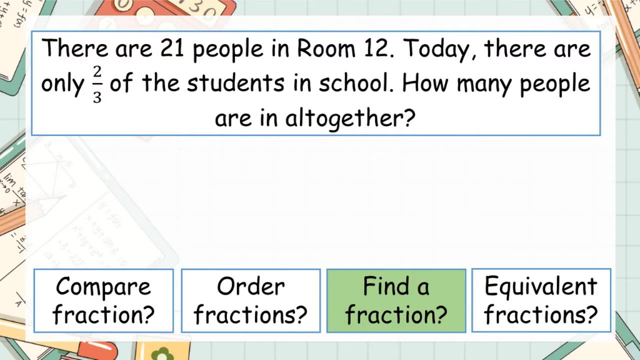 There are 21 people in room 12.. Today, there are only two-thirds of the students in school. How many people are in altogether? Now, this is a finding, a fraction of a set question, Just like the last one we did. but there's one extra step we have to do. 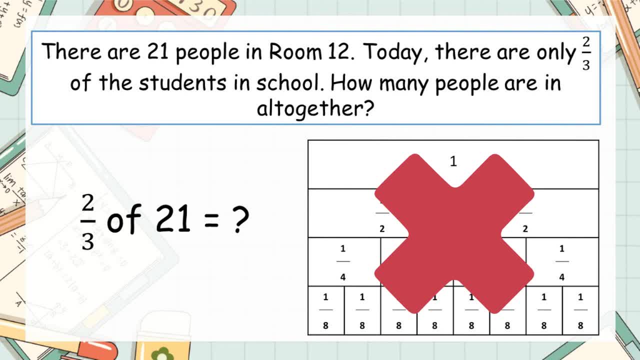 So, first of all, remember, fraction walls are not going to help us here. Instead, we need to do a sum that's going to tell us what two thirds of 21 is. If you want to try and pause the video now and see if you can get an answer, we'll check it in just a few moments, If you've. 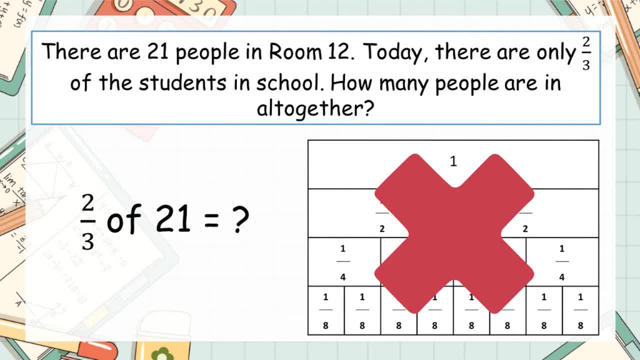 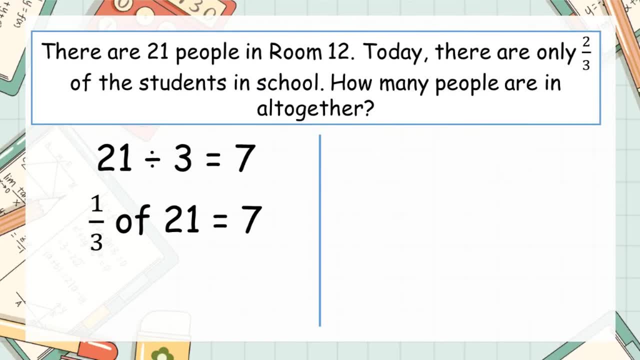 no idea how to do this one. you can just keep watching and we'll talk through it. So there's two ways of doing this again. The easiest way is to use division. Remember, when we want to find a fraction of a set, we divide the total number by the denominator in the 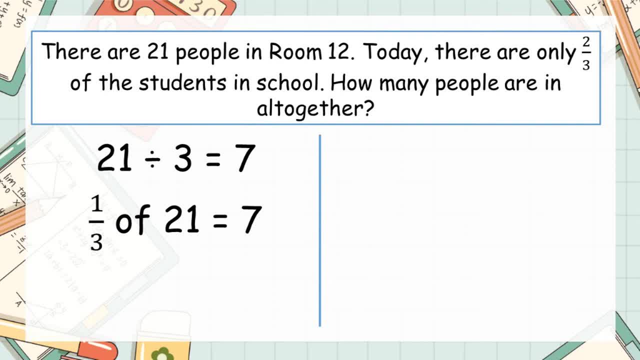 fraction. That's the bottom number. So 21 divided by 3 is equal to 7.. That means that 1 third of 21 is 7.. But we're not looking for 1 third, We're looking for 2 thirds. So 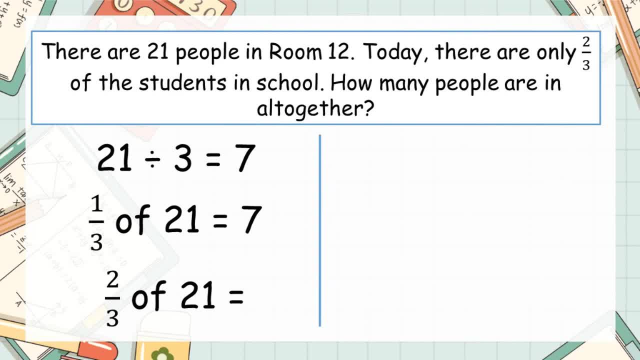 how do you think you'd find 2 thirds if 1 third is equal to 7?? Pause the video and see if you can figure it out. Well, if 1 third is equal to 7, 2 thirds is going to be equal. 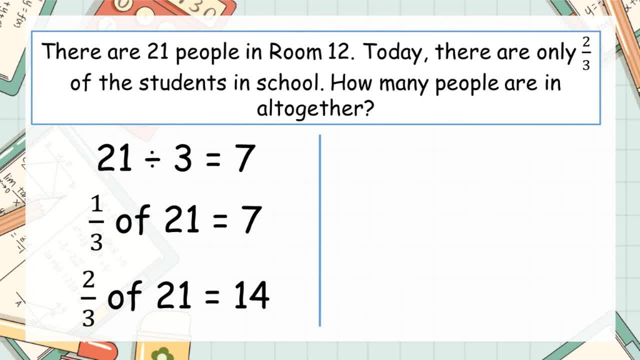 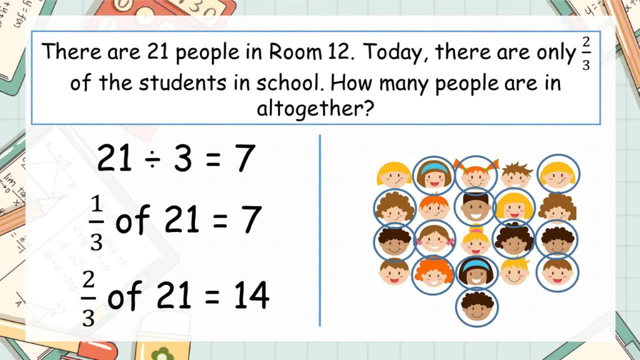 to 14.. Did you get that correct? The other way of solving this is to draw a picture to help us. We could draw the 21 people who are in the class and mark 2 thirds of them. The way we would do that is count up 1,, 2,, 3 and mark 2 people. 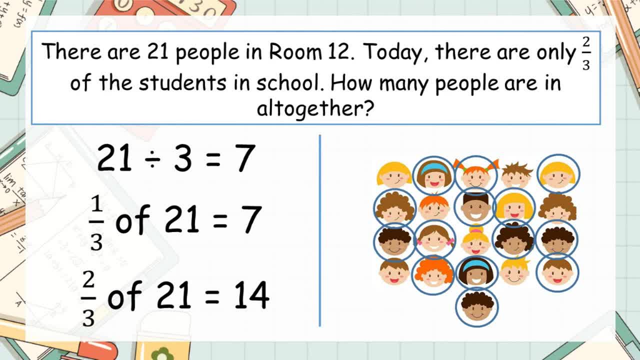 out of 3.. Not 1 person out of 3, like we've been doing before, but 2 people out of 3.. This is because our numerator in our fraction is 2 this time, not 1. We keep on doing that. 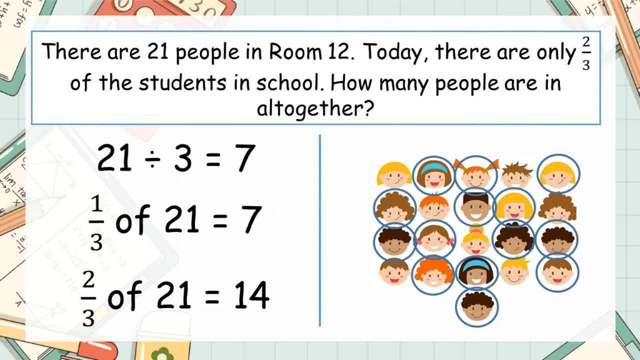 counting up 1,, 2,, 3, and 2.. 1,, 2,, 3, and marking 2 of them. 1, 2,, 3, and marking 2 of them until we've completed the. 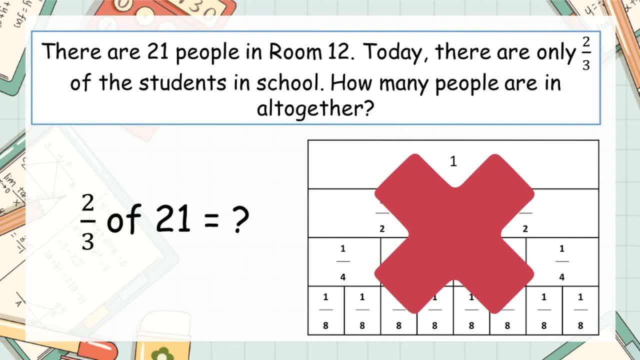 So, first of all, remember, fraction walls are not going to help us here. Instead, we need to do a sum that's going to tell us what two thirds of 21 is. If you want to try and pause the video now and see if you can get an answer, we'll check it in just a few moments. 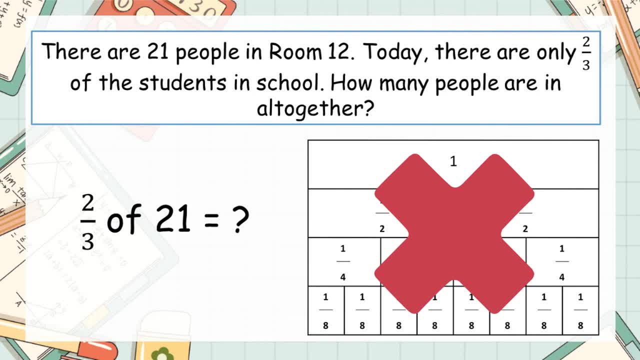 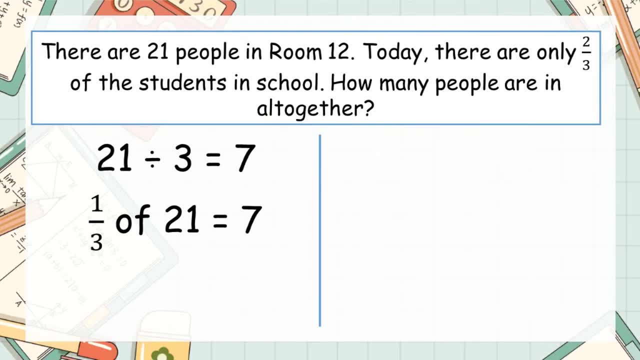 If you've no idea how to do this one, you can just keep watching and we'll talk through it. So there's two ways of doing this. again, The easiest way is to use division. Remember, when we want to find a fraction of a set, we divide the total number by the denominator in the fraction. 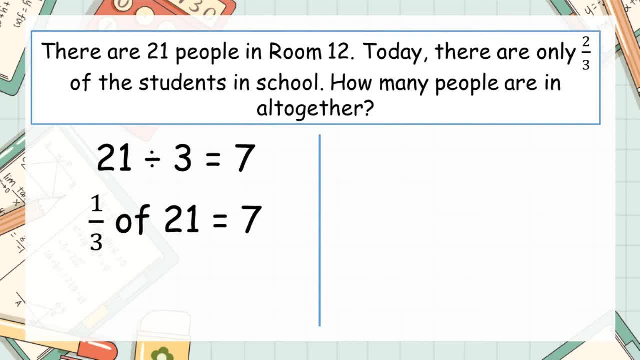 That's the bottom number. So 21 divided by three is equal to seven. That means that one third of 21 is seven. But we're not looking for one third, We're looking for two thirds. So how do you think you'd find two thirds if one third is equal to seven? 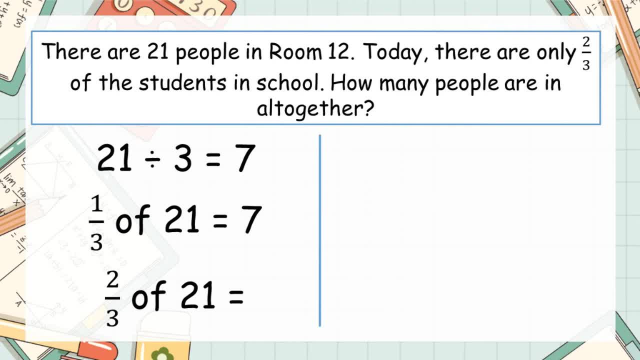 Pause the video and see if you can figure it out. Well, if one third is equal to seven, two thirds is going to be equal to 14.. Did you get that correct? The other way of solving this is to draw a picture to help us. 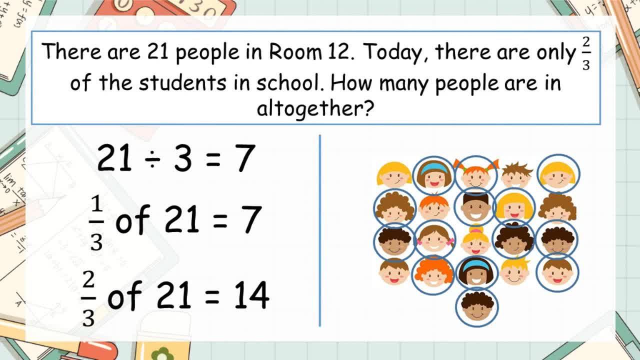 We could draw the 21 people who are in the class And mark two thirds of them. The way we would do that is count up one, two, three And mark two people out of three. Not one person out of three, like we've been doing before, but two people out of three. 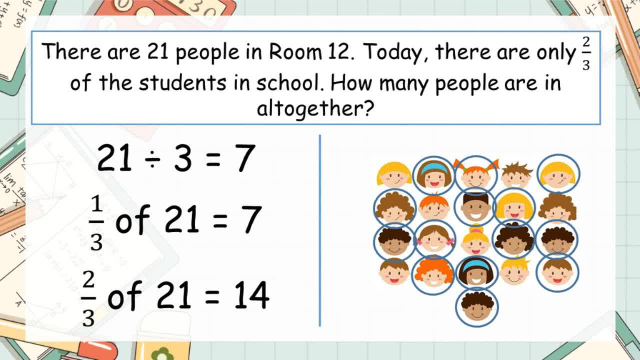 This is because our numerator in our fraction is two, this time, not one. We keep on doing that, counting up one, two, three and marking two of them. One, two, three and marking two of them Until we've completed the whole class. 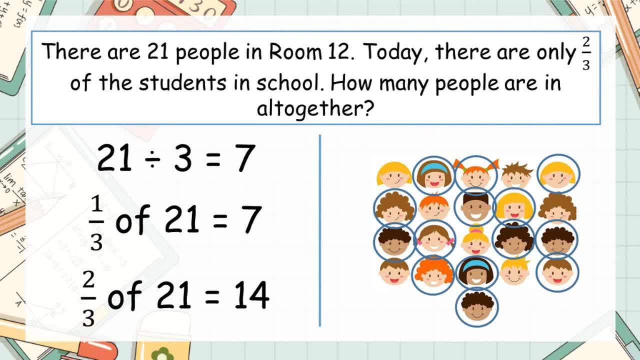 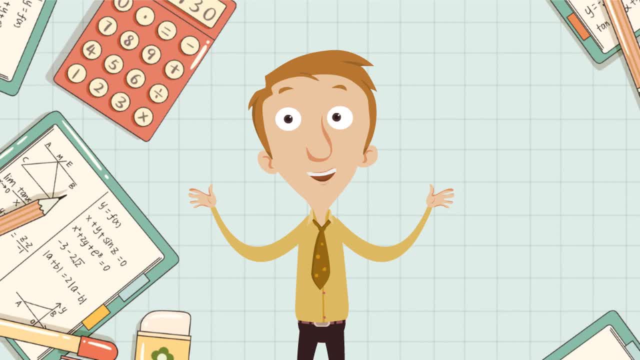 If we do that and count up the marked people, there's going to be 14 of them, Just like when we did the division way. Because those types of questions are particularly difficult, Let's do one more of them to see if you can crack the code. 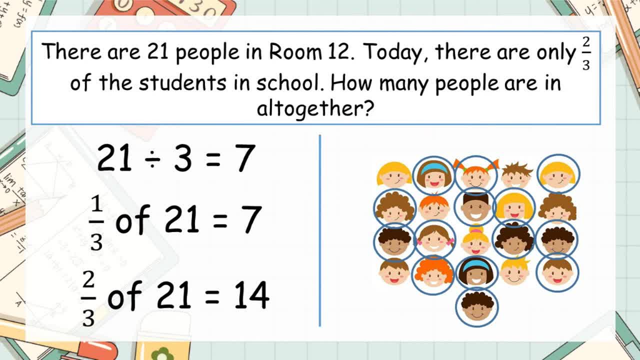 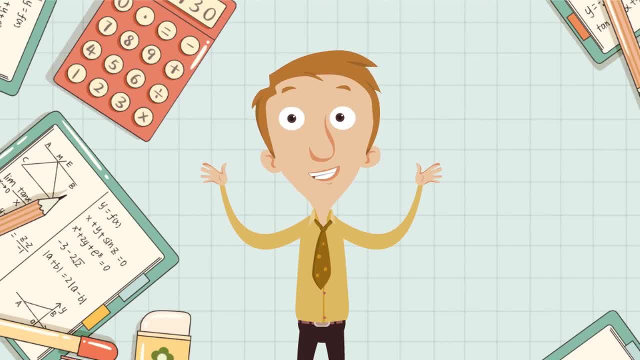 whole class. If we do that and count up the marked people, there's going to be 14 of them, just like when we did the division way. Because those types of questions are particularly difficult, let's do one more of them to see. 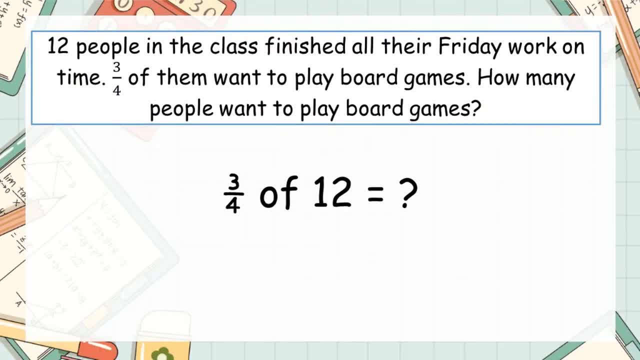 if you can crack the code. 12 people in the class finished all of their Friday work on time. 3 quarters of them want to play board games. How many people want to play board games? So we're looking for 3 quarters of 12.. Can 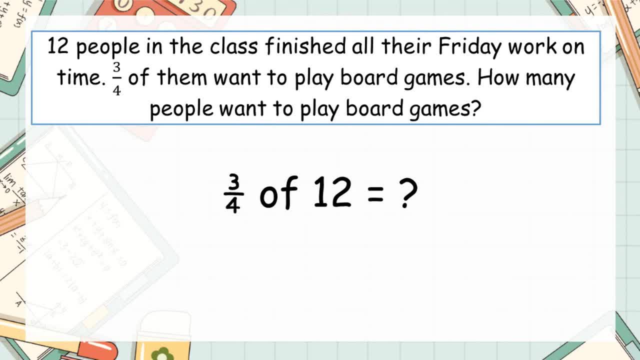 you pause the video and see if you can figure out how many people that would be. Well, if you did it the division way, you would have divided 12 by 4, because that's our bottom number in the fraction. How many groups do we want to make If we did that? 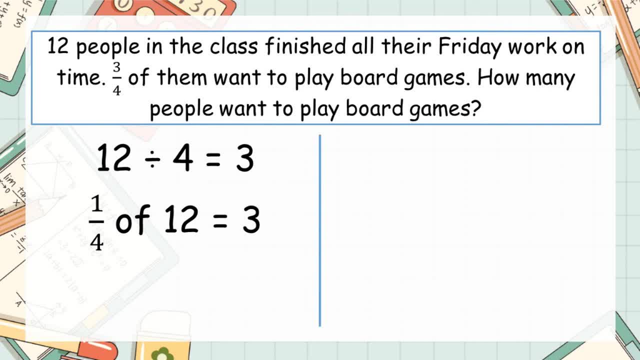 we would find out that 1 quarter of 12 is 12.. 12 is equal to 3.. But we're not looking for 1 quarter, remember. we're looking for 3 quarters of 12.. So if 1 quarter is 3, how many would 3 quarters be? Pause the video and give it. 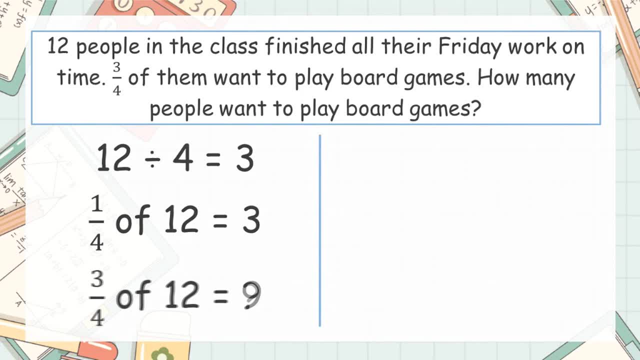 a try. Well, the answer would, of course, be: 9 people want to play board games. 3 quarters of 12 is 9.. If we drew a picture, it would look like this: We would draw out the 12 people. 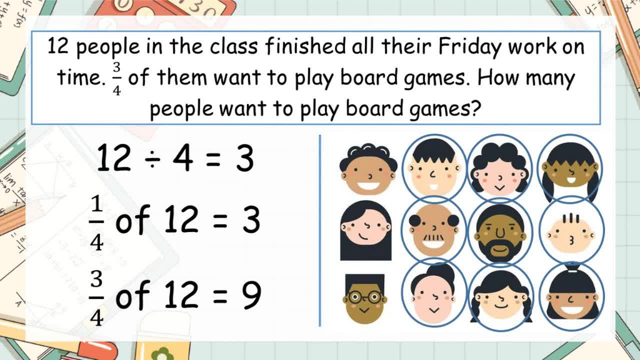 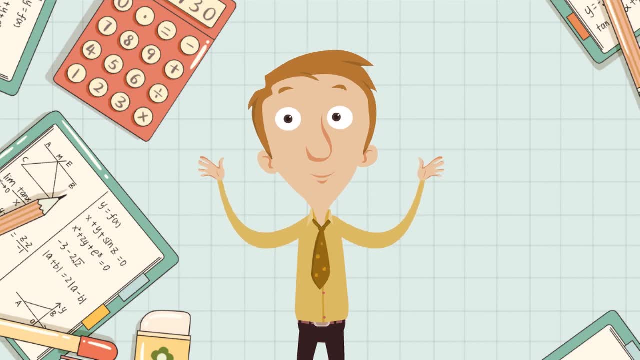 and we would mark 3 out of every 4 people. So we count 1,, 2,, 3,, 4, and mark 3 of them, Because our numerator is 3, and our denominator is 4.. Word problems are tricky and when you add fractions into the mix, you're bound to find: 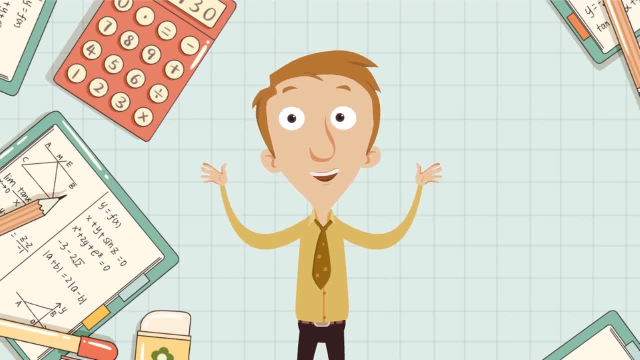 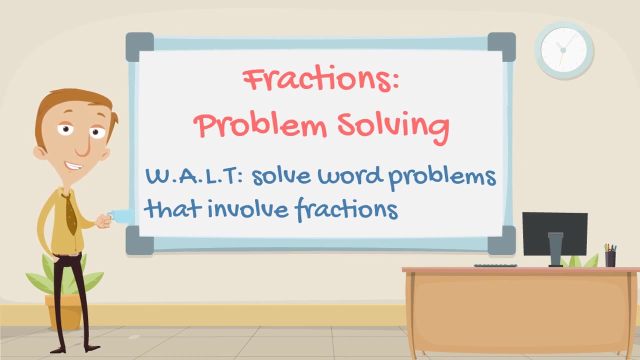 some challenging problems ahead of you, So don't worry. if you need to watch the video again or if you get a little stuck on some of the word problems, Just let me know and I'll be happy to give you a hand. So our waltz for today's lesson is to solve some word problems that have fractions in. 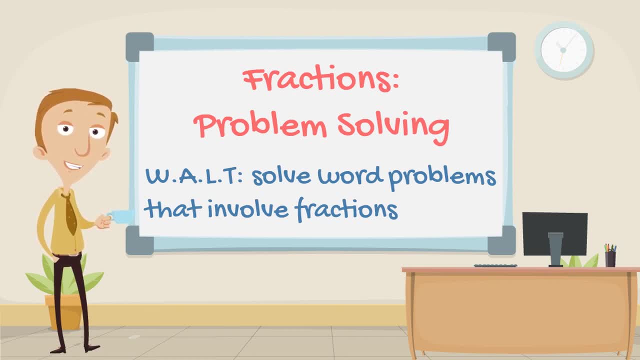 them. You're ready to try that in the activities down below? That's all we have time for today. Until next time, take care.